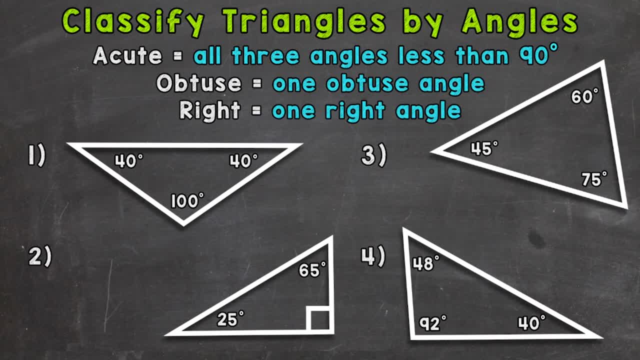 have obtuse triangles- That means one obtuse angle within the triangle. And then, lastly, right triangles- That means a triangle with one right angle. So let's go through four examples of triangles and classify or name them based on their angles, to get a better idea of what all of those 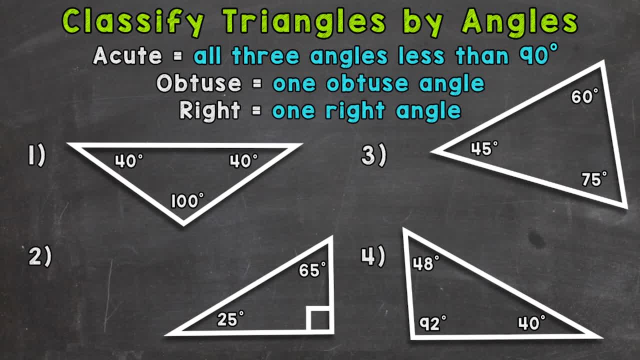 types of triangles look like- And we'll start with number one, where we have a triangle with a 40 degree angle, another 40 degree angle and then a 40 degree angle, And then we have a triangle, 100 degree angle. now there are two acute angles there, but for a triangle to be an 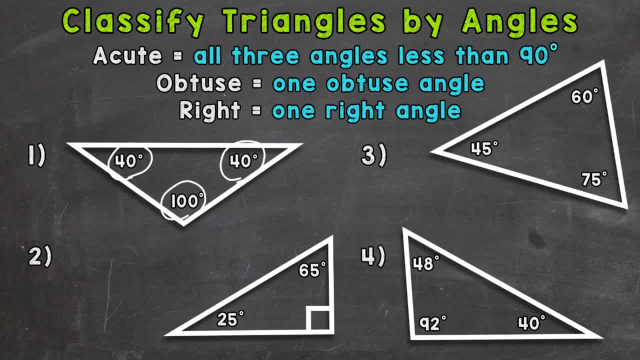 acute triangle, all three have to be less than 90. this 100 degree angle right here is an obtuse angle. it's greater than 90 degrees. so if a triangle has one obtuse angle it's automatically an obtuse triangle. so number one, this would be an 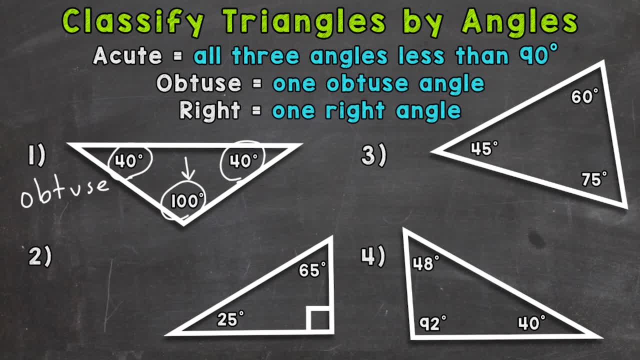 obtuse triangle. number two: we have 25 degrees, 65 degrees and then this signifies a 90 degree angle. so we have a right angle within that triangle. so this is an example of a right triangle. number three: we have 45 degrees, 60 degrees and 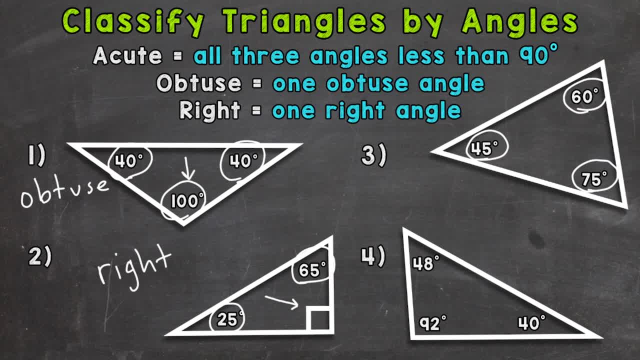 75 degrees. so 45 degrees, 60 degrees and 75 degrees. so all three angles are less than 90 degrees. that means this is an acute triangle. and then, lastly, number four: we have 48 degrees, 40 degrees and then 92 degrees. 92 degrees, that angle is obtuse. it's close to 90. it's close to a right. 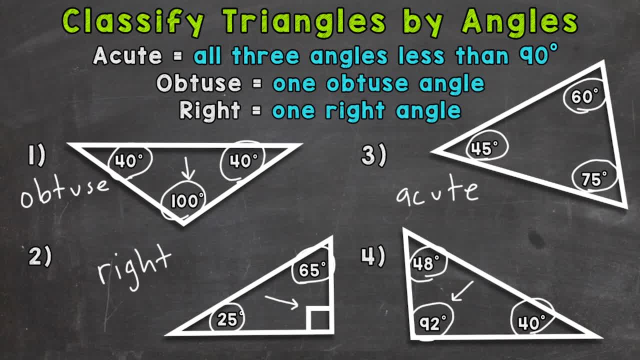 angle, but it is greater. so this is an obtuse triangle, because 92 degrees that angle is an obtuse angle. one obtuse angle equals an obtuse triangle, so number four: obtuse. so there you have it. there's how you classify or name triangles based on their angles. we have three options.